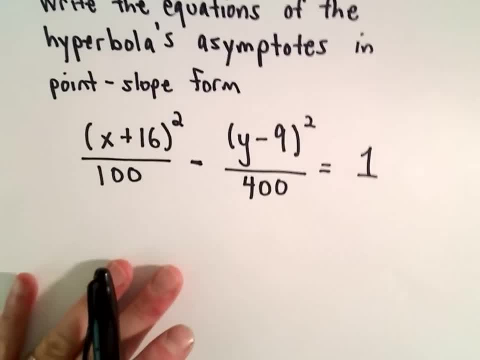 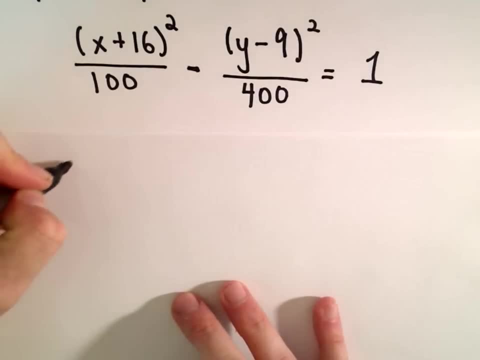 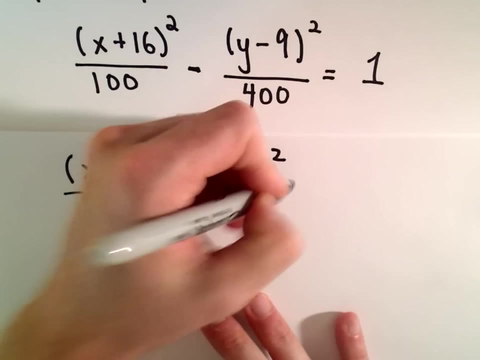 of writing things in a proper form and just knowing some corresponding formulas, So kind of the formulas that we're going to use. we're going to write the hyperbola in the form: x minus h, quantity squared over a squared minus y minus k, squared over b squared. 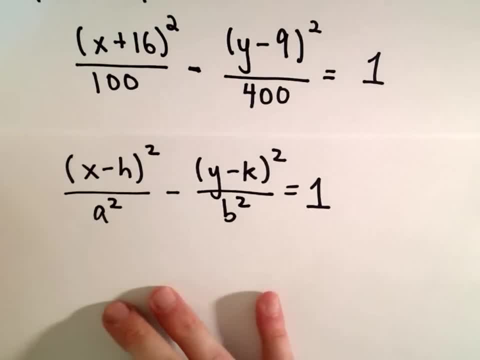 equals 1.. And the idea is, once we write it in this form, this standard form, it says the asymptotes. It says the asymptotes, The asymptotes are going to be of the form: y minus k equals positive and negative. b over 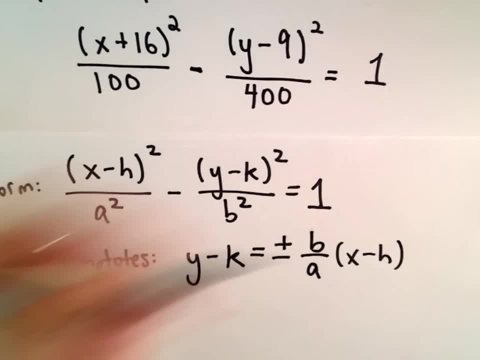 a times x minus h. Okay, so again, what I need to do is I need to figure out a value for k, I need to figure out a value for b, I need to figure out a value for a and I need to figure out a value for h. 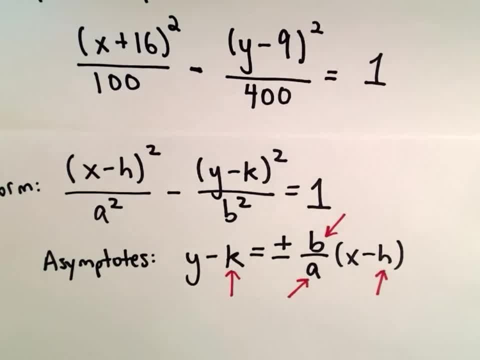 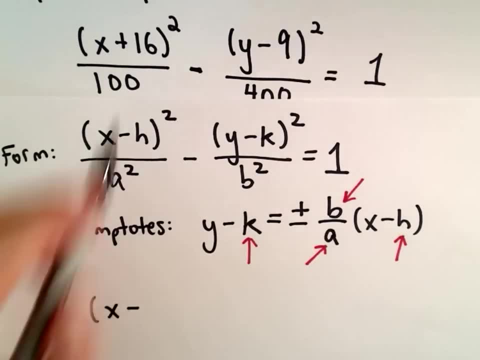 All right, well, let's do that. Okay, So I can rewrite this. So it says we're going to write it as x minus something, So x minus. well, we want it to be equivalent to x plus 16.. So we can write it as x minus negative 16, well squared. 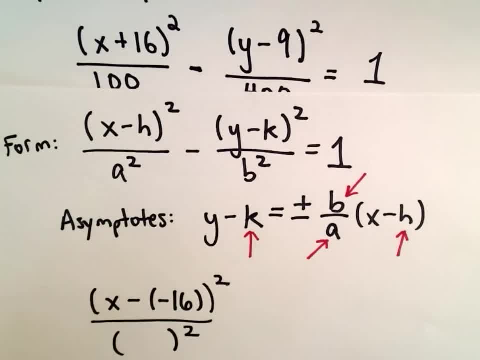 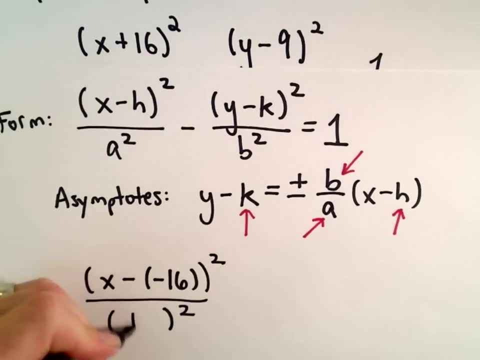 I want to write the denominator as some number squared. Well, I want that number to equal 100.. Well, what number squared is going to be 100? and you could say: well, hey, it could be negative 10.. values be positive. So we're going to use positive 10 squared, And then we've got well. 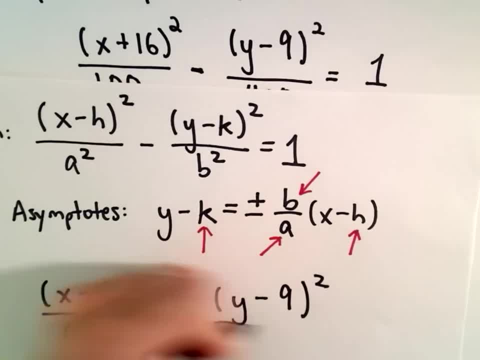 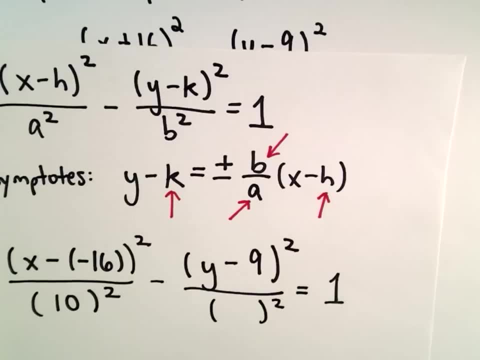 we've got y minus 9.. We can leave that part alone. This is all over 400.. Again, I want to write that as a number squared, a positive number being squared. Well, we can write 400 as 20 squared. So now I've got all my values. okay, It says this is going to be our value. 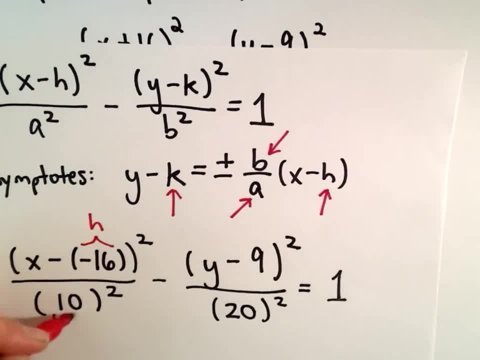 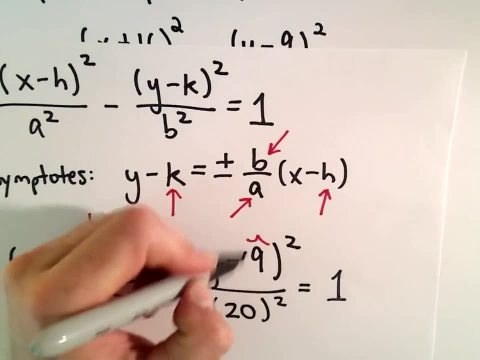 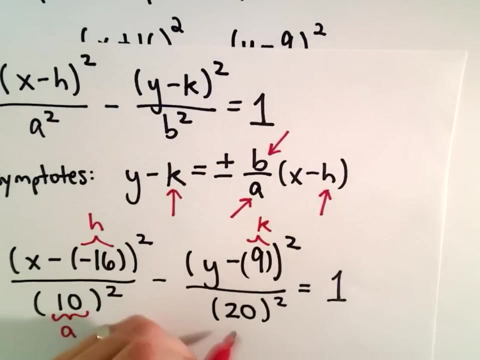 for h. h is going to equal negative 16.. It says 10 is going to be our a value. It says positive 9.. Again, we kind of forget about the negative, So we could write this as y minus 9.. Okay, so that's going to be our k value, And then 20 is going to be our b value. 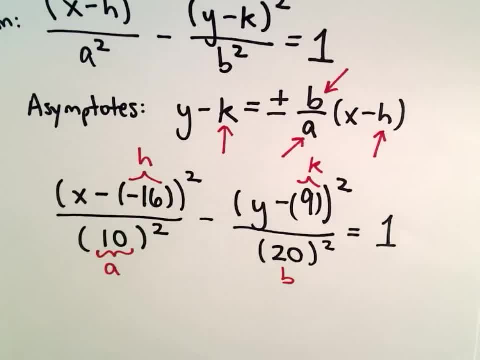 So I'm just going to fill that in and we'll have our asymptotes. So it says our asymptotes will be y minus k, which is 9, equals positive or negative b over a. So again we said b had value 20. a was equal to 10. Then we do x minus the. 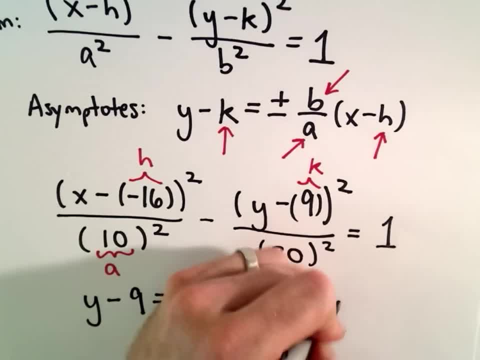 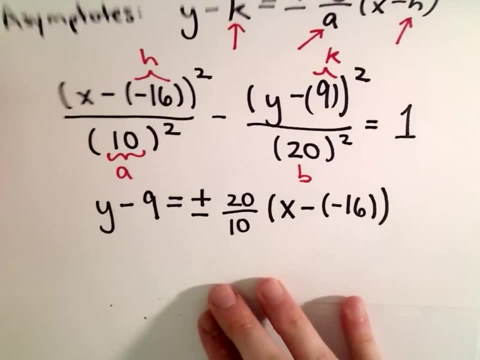 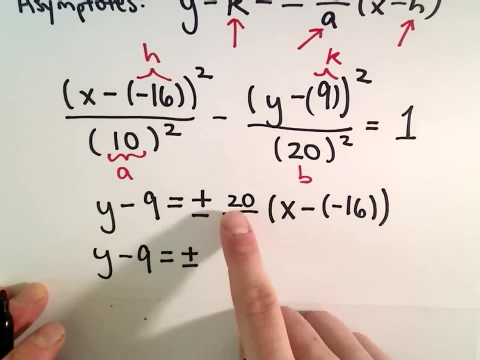 h value. So the h value is negative 16.. And of course we could simplify this down just a little bit, But now we've done everything, So it's just kind of again just you know, just writing things in the proper form and just knowing formulas. So 20 over 10 is going. 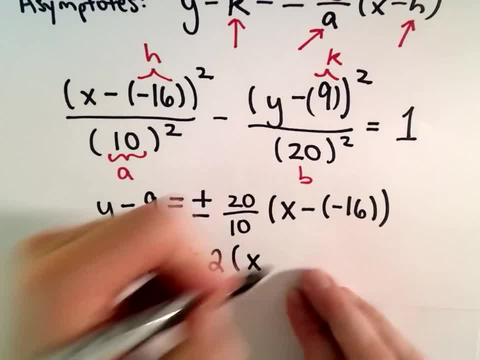 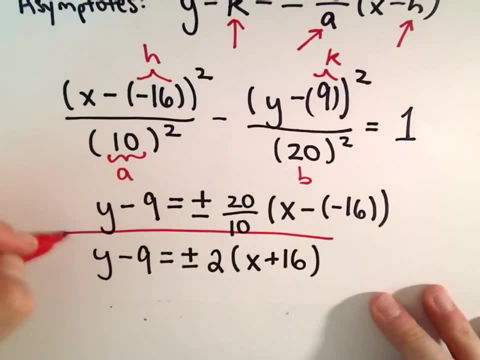 to be 2.. x minus negative 16 will be x plus 16.. And now we have our asymptotes. 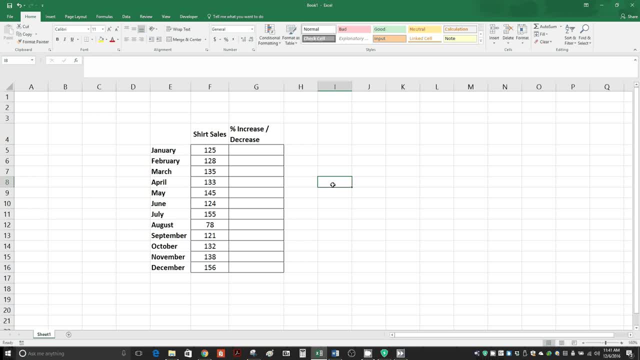 Today we're going to calculate the percent increase or decrease for data in Excel. I made some mock data here for January through December for shirt sales, Alright, so we can't actually calculate any data for January because we don't have any previous data. The very first piece of data will not have a percent. 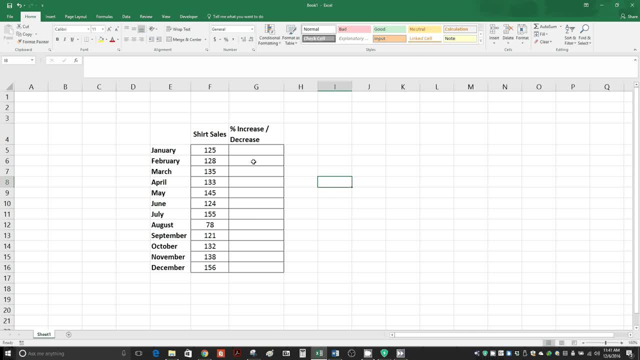 increase or decrease. So we'll start with February. So I'm clicking the cell for February, We're going to type the equals symbol. Then we're going to click on the shirt sales for February. Then we're going to hit the divided by key, which is near the bottom part of. 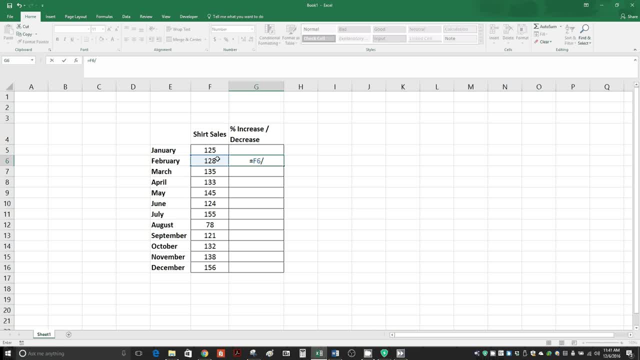 the keyboard on the near the right shift button, Then we're going to click on the shirt sales for January, and then we will simply subtract one, So minus one. So this is how your formula is going to look: Equals February, or, in your case, will be: 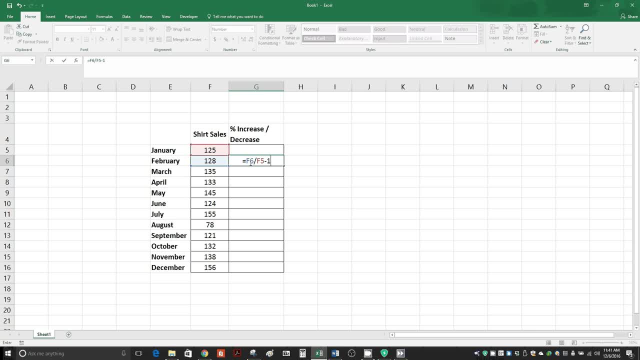 like the new piece of data divided by January, or, for you, be the previous piece of data. So we're going to hit minus one and then hit enter, Alright. so you see we have a 0.02 or two percent increase. Now most people don't like seeing it in decimal form. They want to see it in.